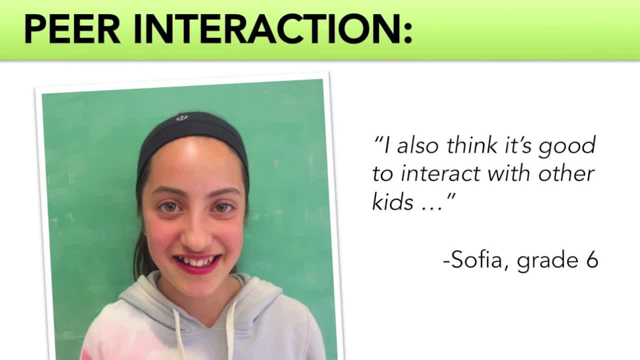 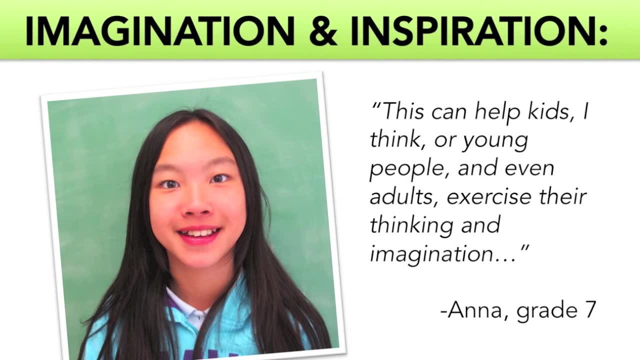 to people, just ask you a question and then just share your own ideas about what you think. personally, I strongly agree with Sophia, because most of the time in the classroom we don't get to sit in a circle like this and just discuss ideas about deep, really deep questions and 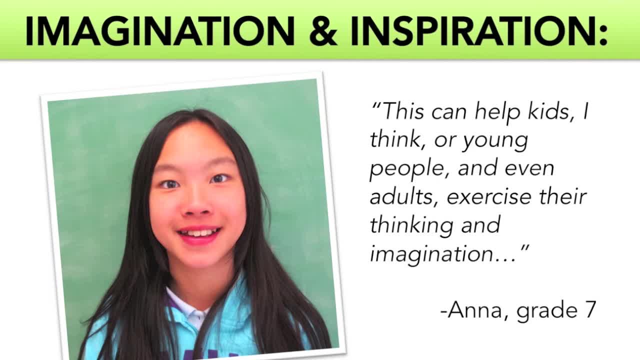 this can help kids, I think, or young people and even adults exercise their thinking and imagination, because sometimes the best ideas just come to your mind when you're just sitting there and you listen to other people and you get inspired and you get your own ideas. 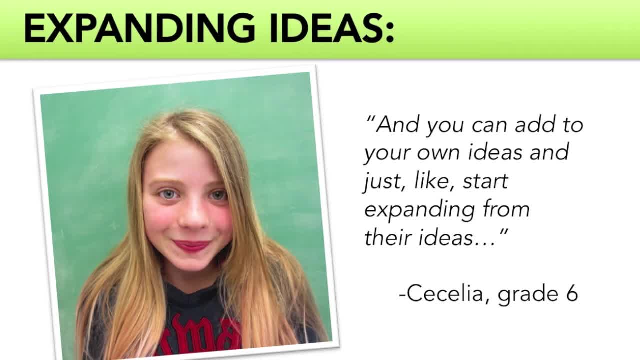 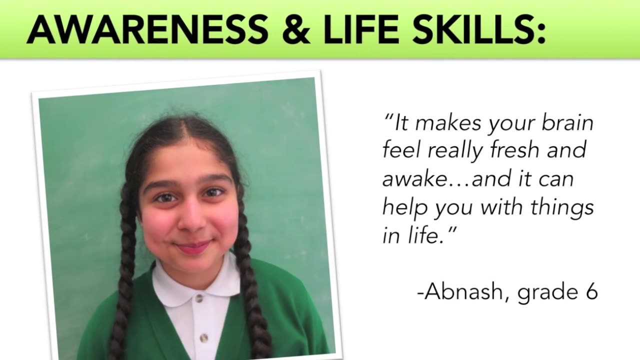 I think it's good for people because, like, you can like get other ideas from people and it's like you learn from them and you can add to your own ideas and just like start expanding from their ideas. It makes your brain feel really fresh and awake and it can it can like help you improve. 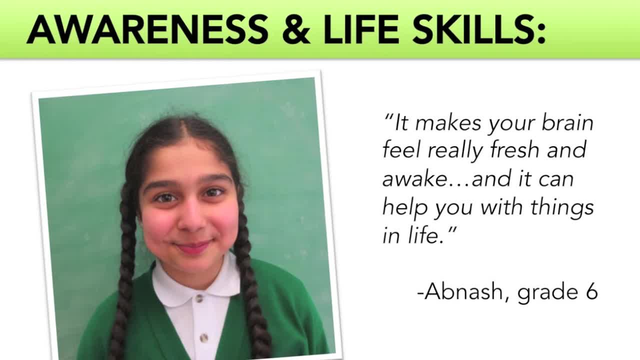 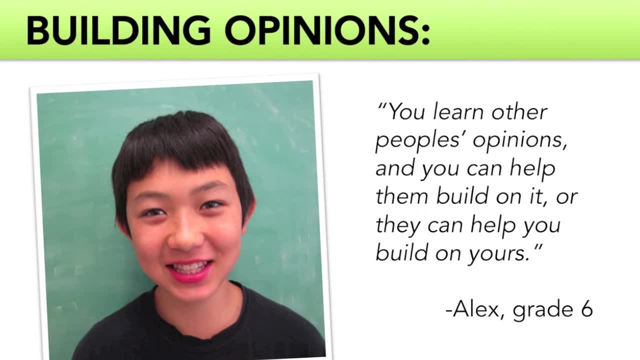 in other things, as it like, helps improve your imagination and it can help you with things in life. I think it's helpful. I think it's helpful Because when you're in a group talking, you learn other people's opinions and you can. 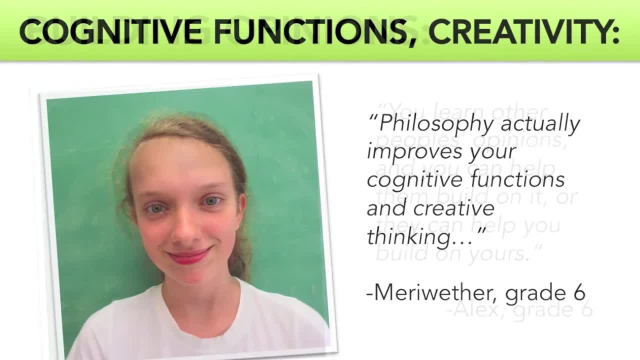 help them build on it or they can help you build on yours. On a more scientific view, talking to other people and doing philosophy actually improves your cognitive functions and creative thinking, so you're able to think about things more and share your opinions and do many other things that you wouldn't be able to do with. 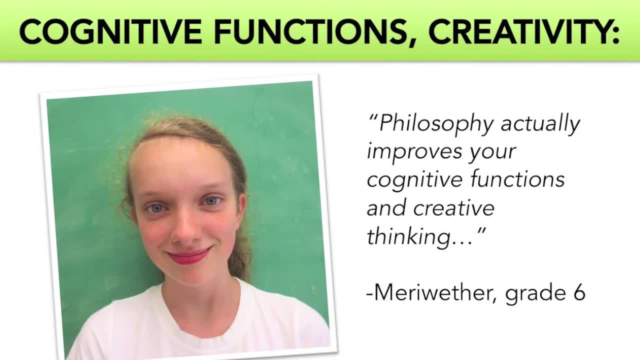 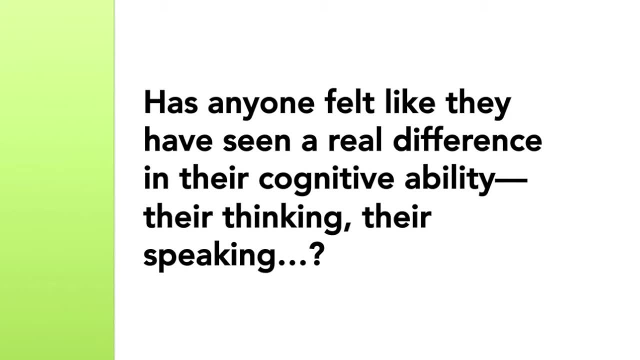 that you wouldn't be able to do as easily Without philosophy. Has anyone felt like they have seen a real difference in their cognitive ability, their thinking, their speaking? I think I've grown from this because sometimes, when people like if someone used to ask. 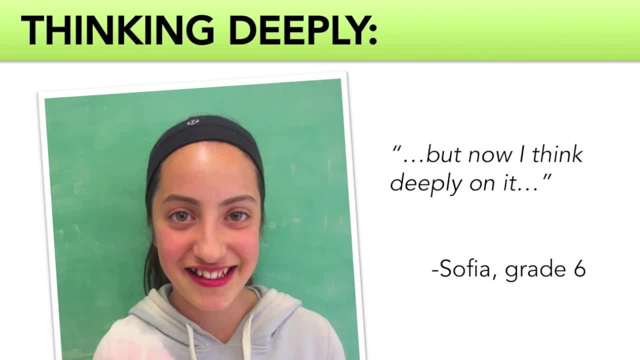 me a question. I'd just say the first thing that comes to my mind, but now I think deeply on it and it you get to express more things and you realize, like more about what the question. I guess I've changed because I used to be really happy. 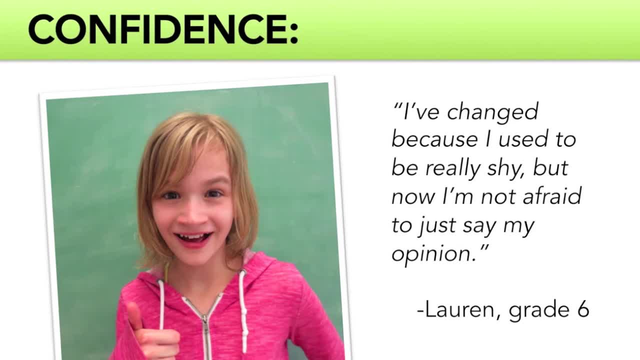 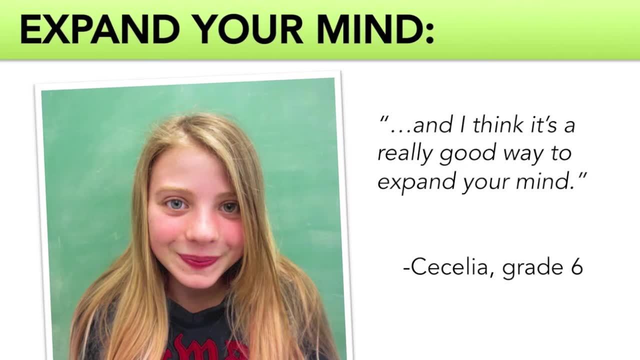 I used to be really shy, but now I'm not afraid to just say my opinion. I think I've grown a lot from this because, like last time, someone said something that I thought was like really smart. so then I like kept thinking about it and I like 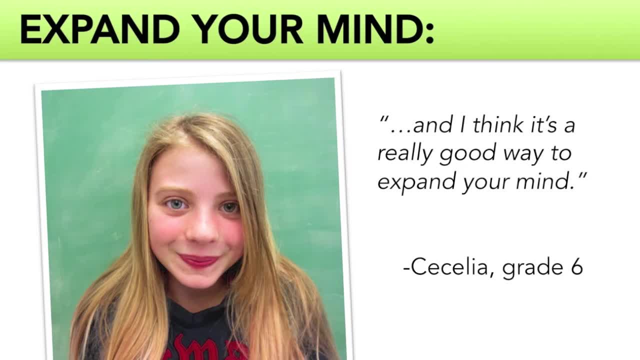 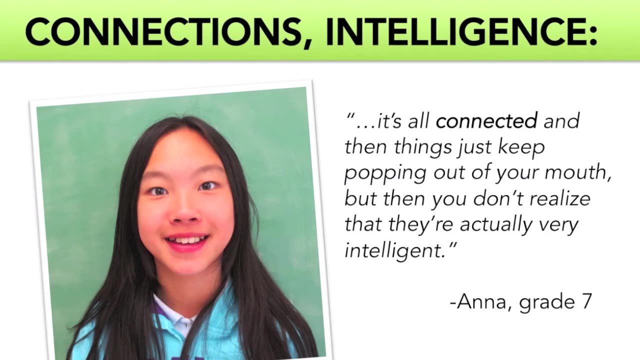 just couldn't get it out of my mind and I just kept like thinking it over at night and stuff, and I think it's a really good way to expand your mind. I agree, I think that we have, we can learn and grow from this, because before it used to be like 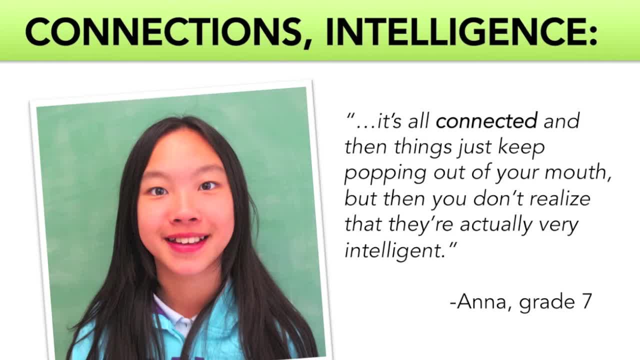 when, like when someone asked me a question, I would just say a really obvious answer, and now I- and before it would usually take some time for me to think and get all the ideas out- but then now it's like when you're talking like one idea leads to another and 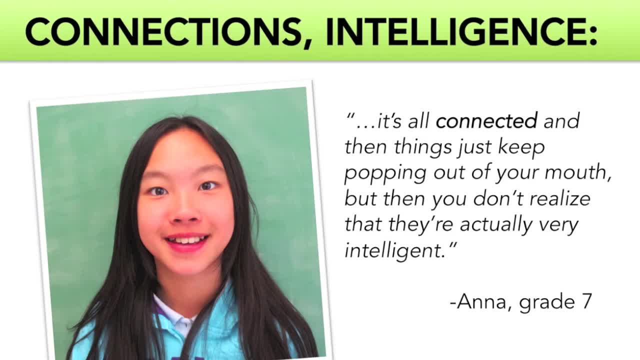 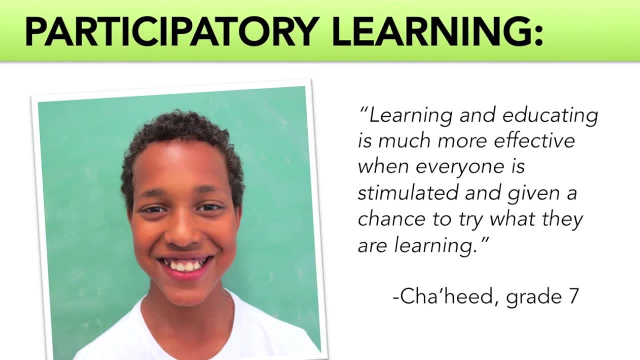 then it's all connected and then things just keep popping out of your mouth, but then you don't realize that they're actually very intelligent. Okay, I think that I have learned and benefited really well from this, and I found that being stimulated and being able to talk and express yourself is a very effective way of learning. 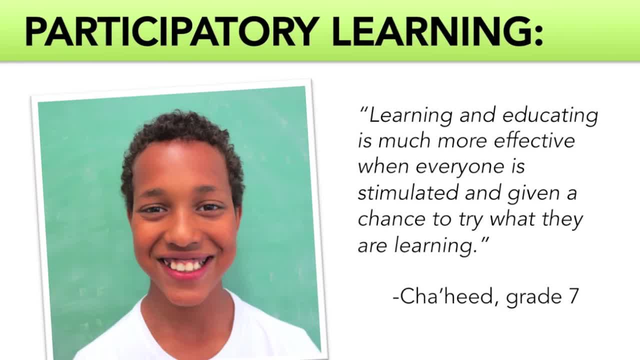 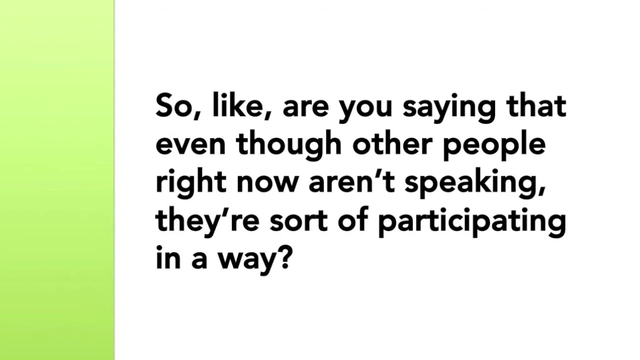 instead of in a classroom where you're doing math and two or three people might go up and try it. when we're learning a new concept, I feel that learning and educating is much more effective when everyone is stimulated. So like are you saying that, even though other people right now aren't speaking, they're 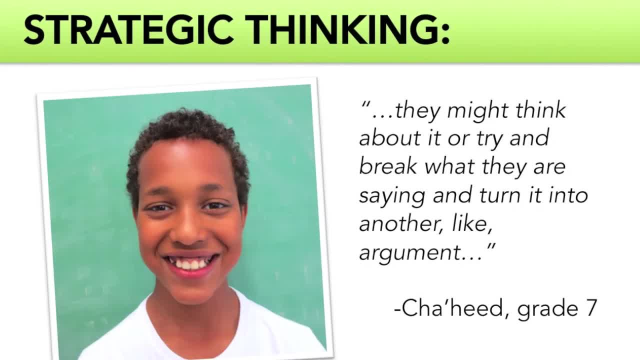 sort of participating in a way. Yes, because when they hear someone say something, they might think about it or try and break down what they're saying and turn it into another like argument or something against someone else. I think I have changed. 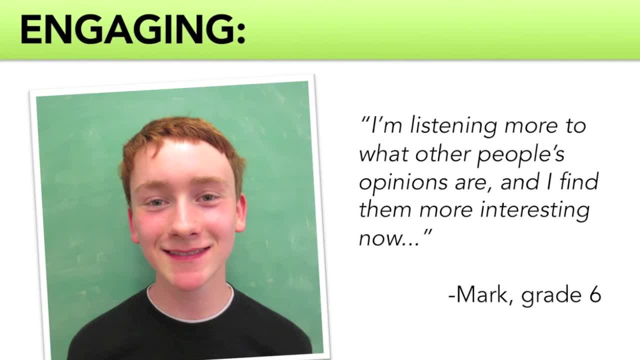 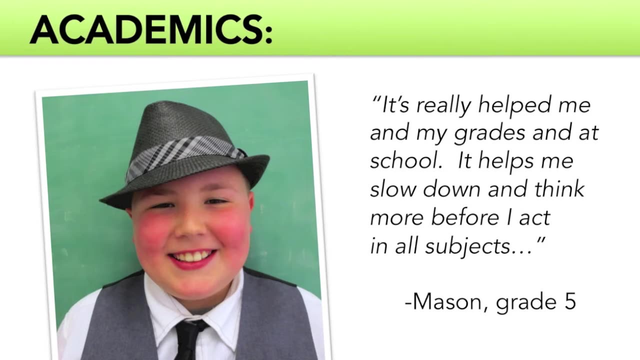 I think I have changed. I am listening more to what other people's opinions are and I find them more interesting now as I learn more about philosophy. It's really helped me in my grades in that school. It helps me slow down and think more before I act in all subjects and it has saved me. 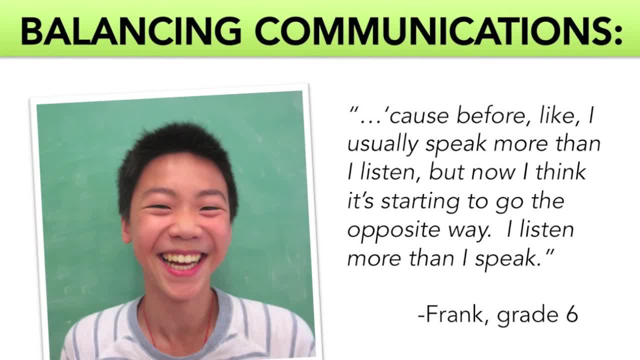 a couple times I agree with Mark, Like well, now I'm more keen to listen than speak, because before, like, I usually speak more than I listen, but now I think it's starting to go the opposite way: I listen more than I speak. 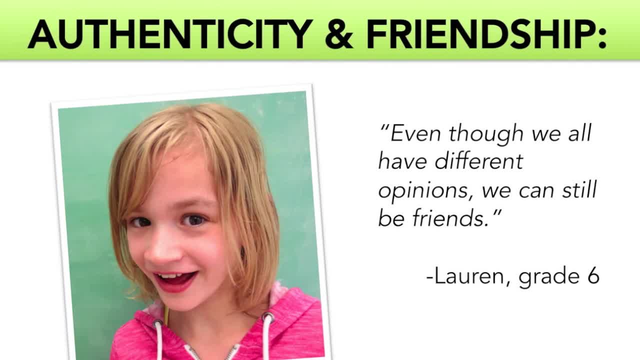 I think philosophy could help everyone, because I've noticed that kids just want to fit in. But with philosophy then they can just not be afraid to be themselves and know that even though we all have different opinions, we can still be friends. I agree. 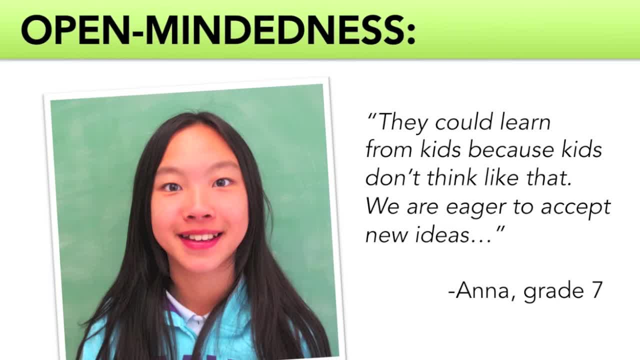 I agree, And I think not just helping kids, it could also help adults, because they've grown to like what they've learned and what their parents have taught them and what their childhood friends think, and then they've grown up thinking that way and it's like they've stuck to those. 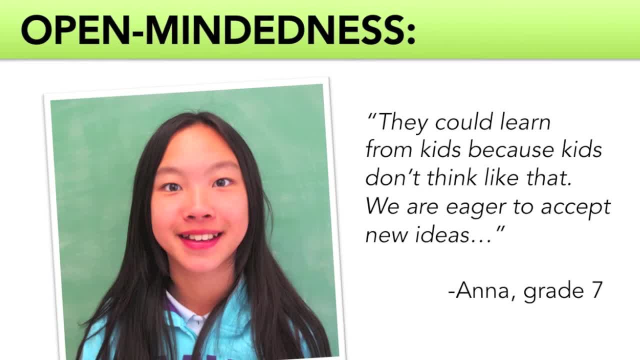 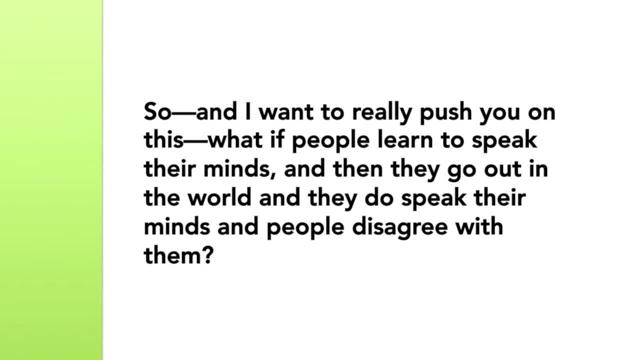 traditions, But then they could learn from kids, because kids don't think like that. We are eager to accept new ideas. So- and I want to really push you on this- what if people learned to speak their minds and then they go out in the world and they do speak their minds and people? 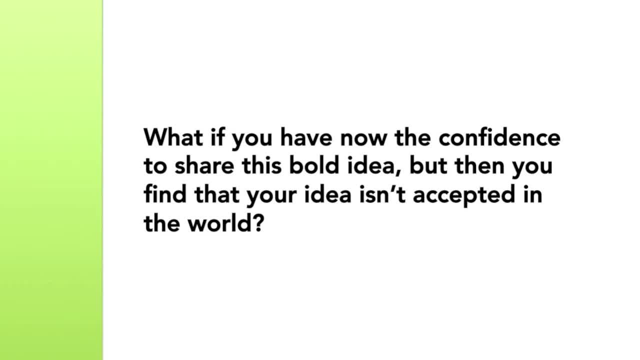 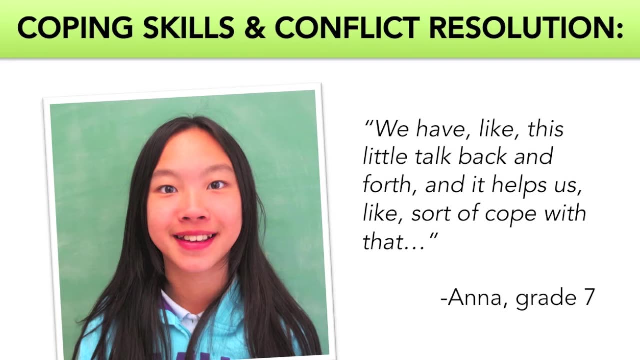 disagree with them. What if you have now the confidence to share this bold idea, but then you find that your idea isn't accepted in the world? That's because that's also what we're learning here in this philosophical group. is that? because when we speak our own ideas, sometimes other people might not agree, and then we 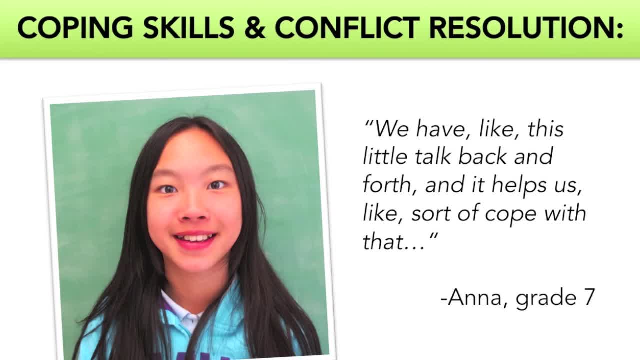 have like this little talk back and forth And it helps us like sort of I don't know cope with that And like for example before when Meriwether was talking and then Mark disagreed with her and then, but eventually they solved that problem and came to terms. 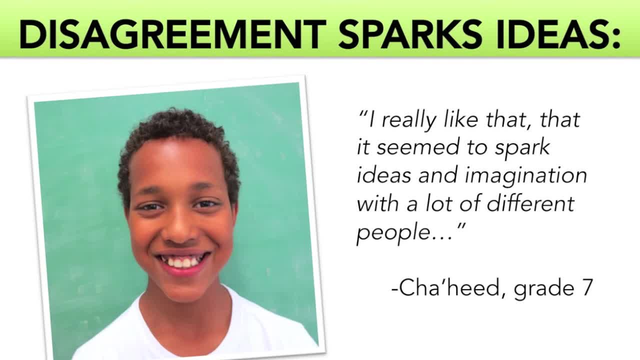 I really liked it when people disagreed with me or like I disagreed with people, like you could kind of see how they were puzzled. I really liked that, that it seemed to spark ideas and imagination with them And I found it a really good experience and really interesting when people were disagreeing. 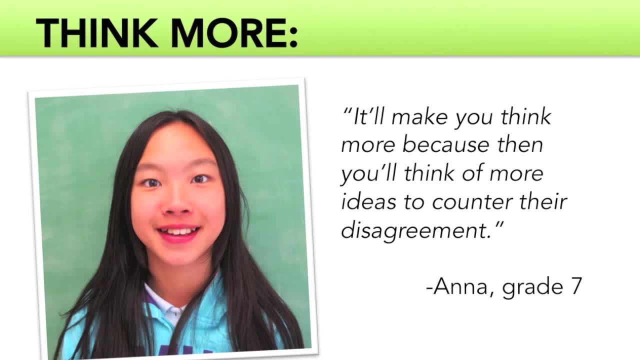 with each other. Hey, that takes courage. I strongly agree with Shahid, because when people disagree with you, they'll make you think more, because then you'll think of more ideas to counter their disagreement. Does it matter the manner in which they are disagreeing? 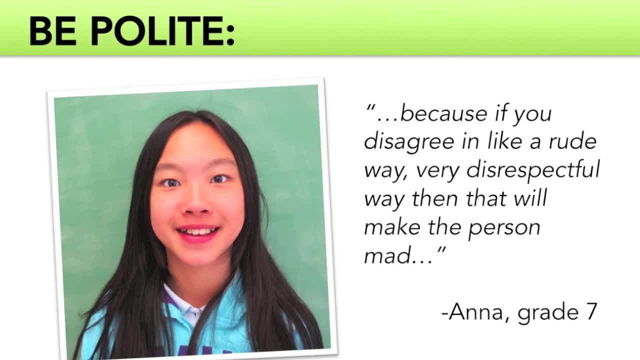 Yeah, because if you disagree in a polite way, then that'll, because if you disagree in like a rude, very disrespectful way, then that'll make the person mad And then they'll like, they'll just they'll come back with a different approach. 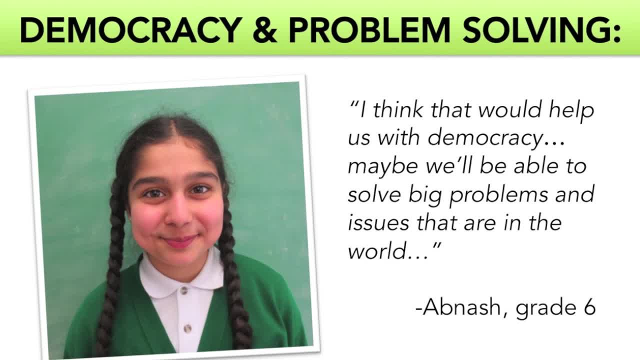 I think that it would help us with democracy because with the future generation I agree with what she said And I think that maybe we'll be able to solve big problems and issues that are in the world because our parents and other adults that are in the world right now they haven't been 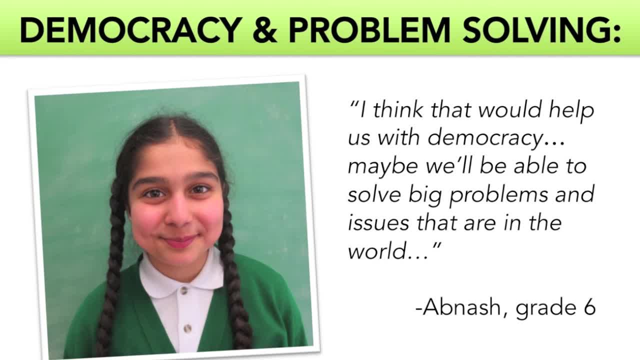 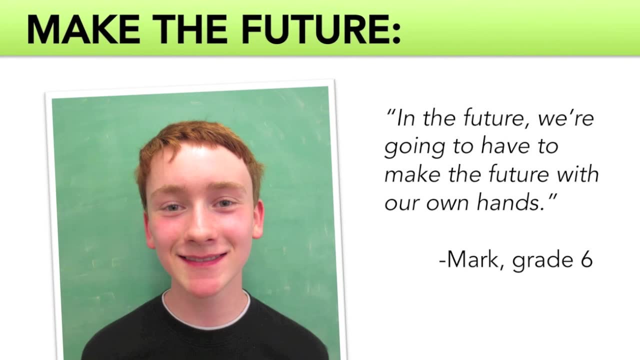 able to solve any problems, probably because they weren't taught Yeah, And so we might be able to think that way, And so we might be able to stop many problems like global warming and other stuff. I agree with Anna's idea because, like she said, children are the future and well. 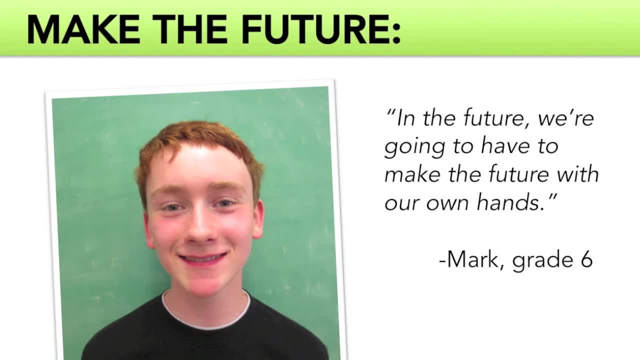 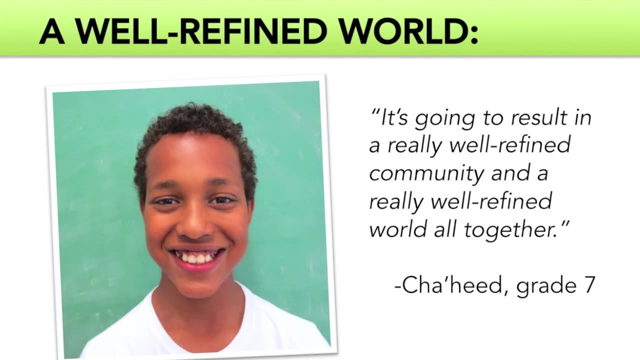 they are, because what's going to happen when all the adults perish And well, in the future, we're going to have to make the future with our own hands. Yeah, I agree with Mark. Right now, kind of what we're doing is picking out flaws with our world today and with adults. 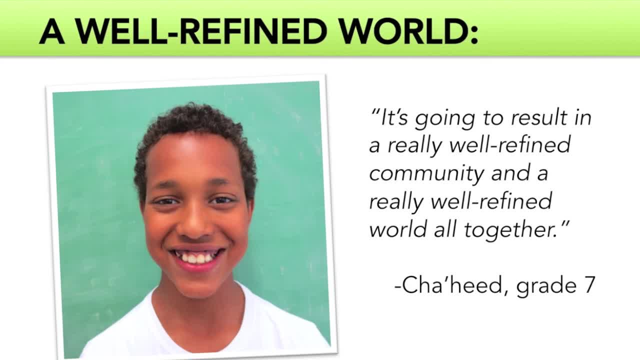 And I think that's a really good thing, because when we become the adults and then we have kids, they're going to learn to think like us. they're going to learn how to pick apart society and the adults and how things work. 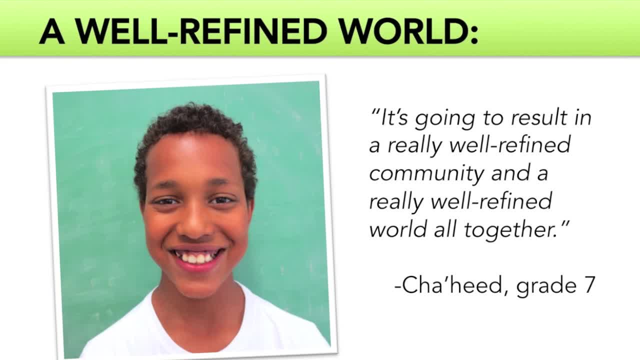 And they're going to be constantly looking and looking for a new way to do things And with people with that attitude, it's going to change, Yeah, And it's going to result in a really well-refined community and a really well-refined world.